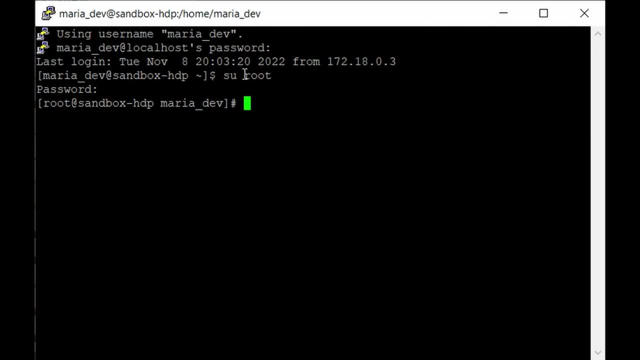 the Kafka is extracted in our sandbox. So you have to just go to the directory as user HDB, Current, And here the directory is Kafka broker. So here, if we just LS, So here are all the directies where we have the bin directory config and all the libraries which are pre. 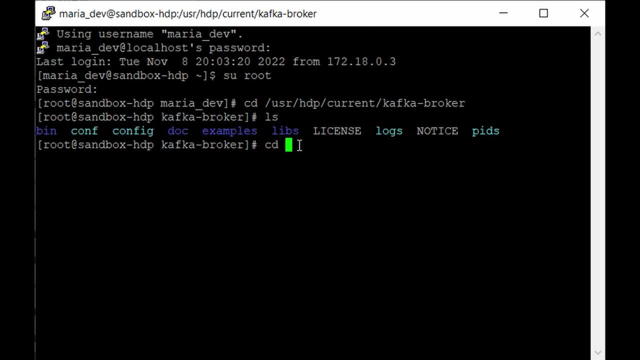 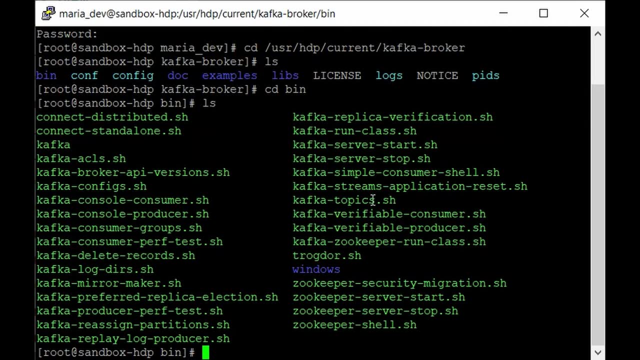 installed in our sandbox, So we just have to go to the bin directory where we'll find all the executable files. So if you give LS, here are all the consumer topics as well as producers scripts ready, So we can just kick it off this predefined shell script to create. 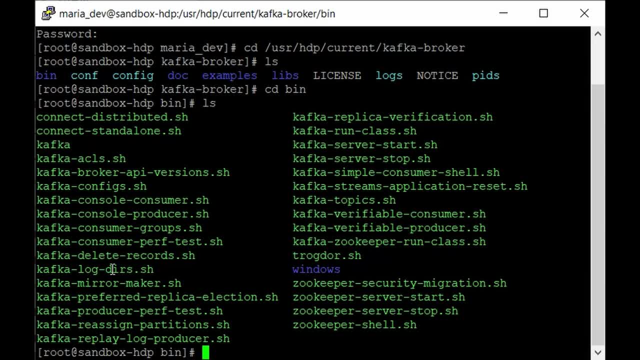 our topics and use the already created shell script to create our personal scripts. So we can just click on the select all And we can see here that we have all the products- consumer and producer application. but first we need the topic in our Kafka cluster. so I hope you already know that topic is nothing, but you can relate it. 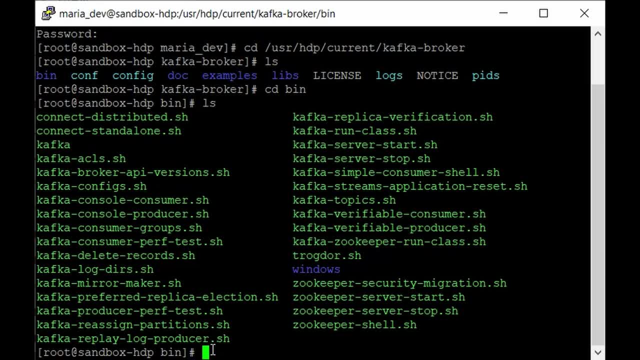 as a table in a relational database, so it stores your data, or you can say the event streams for some particular time period. so, without wasting any time, we'll just create our topic and we can just insert some data into it, just to let you know the power of Kafka and how it ingests data all in real time. so to 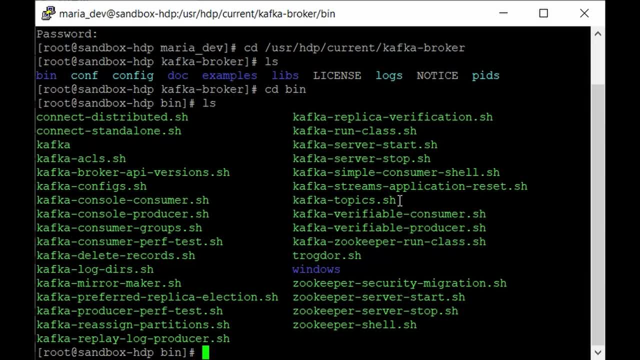 create the topic. we have the file like Kafka topics, dot SH. so to kick off that file, just give like dot slash Kafka topics, dot SH and we have to pass the arguments as create as we are creating the topic and now we need to provide the address for our zookeeper. so I hope you already know that zookeeper is also part. 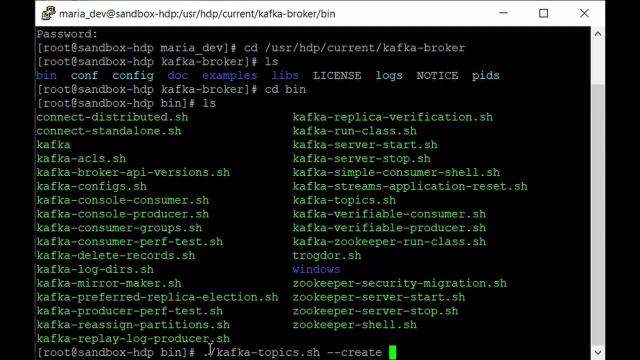 of the Hadoop ecosystem. so you have to mention the address where Kafka can communicate with zookeeper. as you already know, that zookeeper is also a pillar of Kafka architecture. so to give that, just give like zookeeper and zookeepers addresses: sandbox dash HDP dot Hortonworks dot com. so if you are using 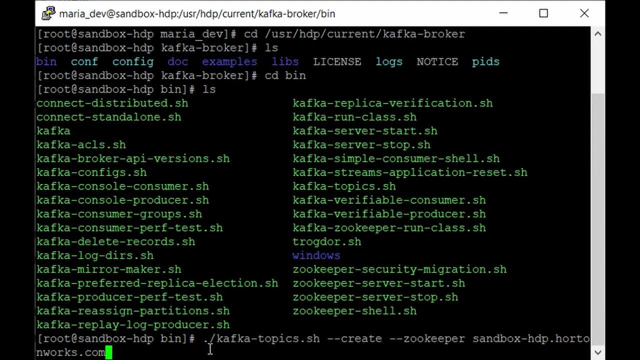 HDP. two point six, point five, then you have to follow the exact command. but if you are using like two point five version, I have given all the commands in the description below. so instead of these zookeeper address, instead of sandbox dash HDP, it's like sandbox dot HDP. so to make sure that you are giving 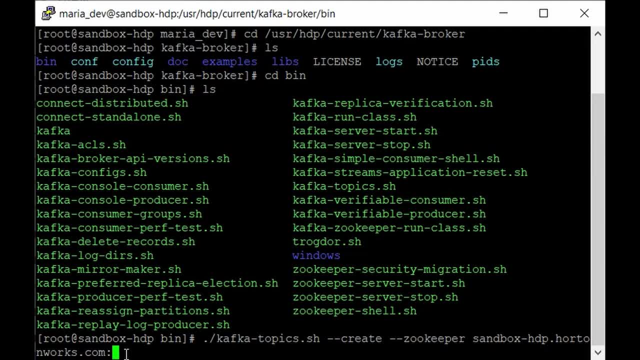 correct address to your zookeeper and it is running at a service two. one eight one zookeeper is available at this port. then you have to do the replication factor. so I hope you already know that replication factor is very important when you're dealing with distributed systems. but here we only have one node. it does not. 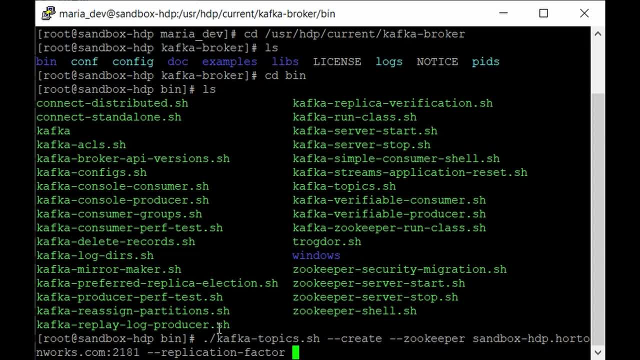 make any sense to give any replication factor beyond one, so we'll give it as one. we have to give the partitions as well. so partitions also we can give one, because we are just messing around to get you the familiarity of Kafka. so just give like one. and we have to give at last the topic name. so give the topic. 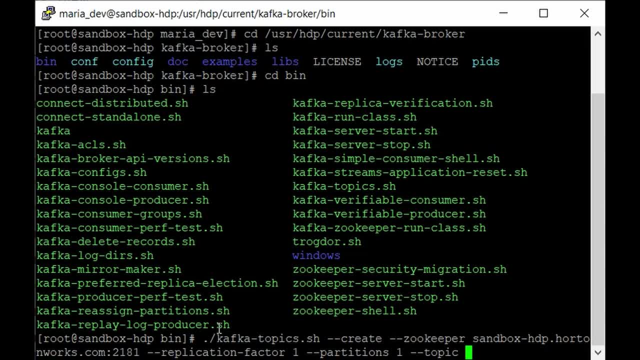 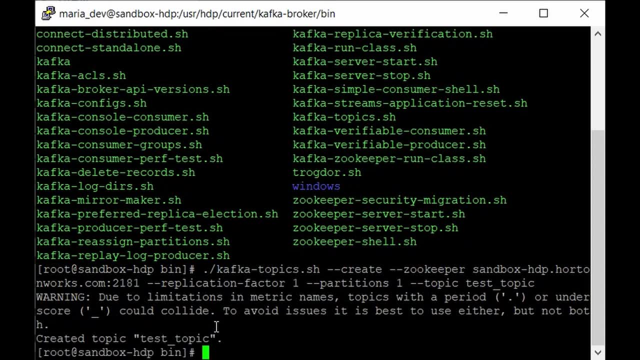 and the topic name is: we can give like test topic. you can give any name of your choice. so if everything looks good, hit enter. so, as you can see, test topic has been created. so just to make sure, we will list all the topics now. so again you have to kick off the same file, kafka topics dot sh. we will. 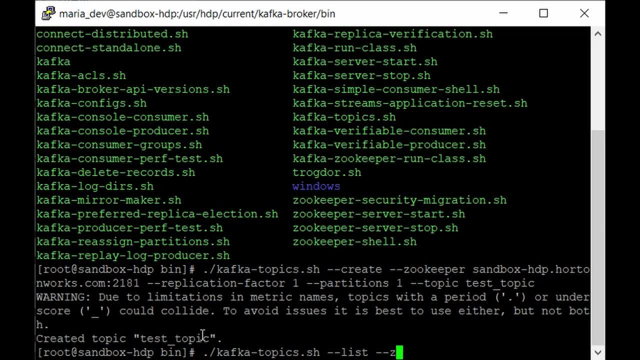 give like list here and also you have to provide the zookeeper address as well. so give like zookeeper again. you sandbox dot HDP dot. Horton works dot com and it is listening to the port. two, one, eight, one and it enter. so this will give you all. 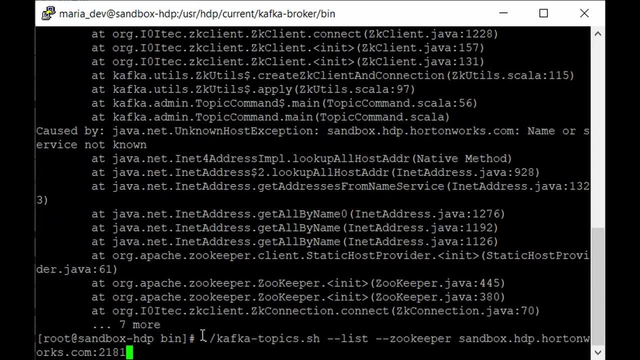 the list of topics present in your Kafka service. yeah, so I made the mistake. so you have to give the zookeeper address of the zookeeper address of your Kafka service. so I made the mistake. so you have to give the zookeeper address of the sandbox dash HDP, not dot. so for a version two, point six, point five, you 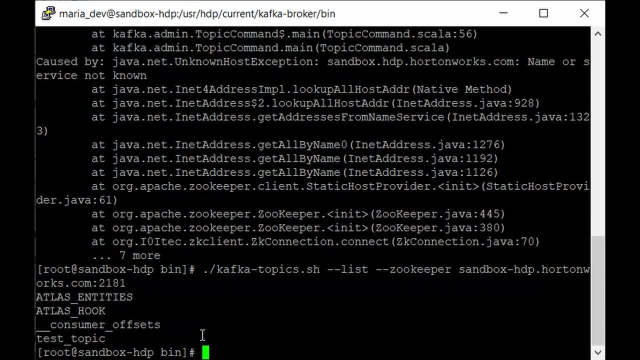 have to give the dash here, so give dash and again rerun it. so, as you can see, these are the topics present on our Kafka cluster. so this atlas, entities, who and this consumer offsets are nothing but already created topics. so here is our test: topics created on our Kafka cluster. so we are ready to inject some. 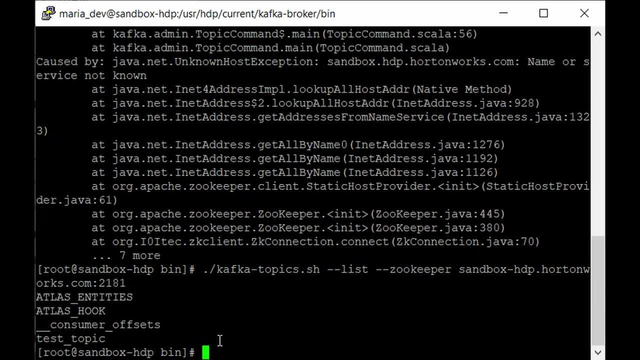 data into it. so for that purpose we need to kick off the consumer application as well as the producer application. so the task of the producer application is to listen to any incoming new data and write it into the Kafka topic, and then consumer then listens to the newly entered data in Kafka topic and displays it for further. 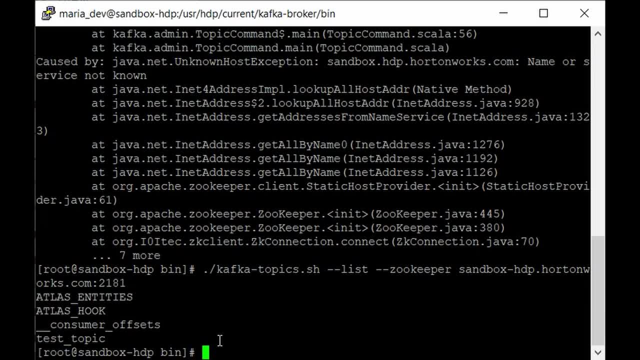 processing. so for this purpose, you will going to ingest some text data directly from the command line. so for that purpose, we need to kick off the producer application, which will produce the data in single command line instance, and will kick off the other command line instance using putty to kick off the consumer application, which 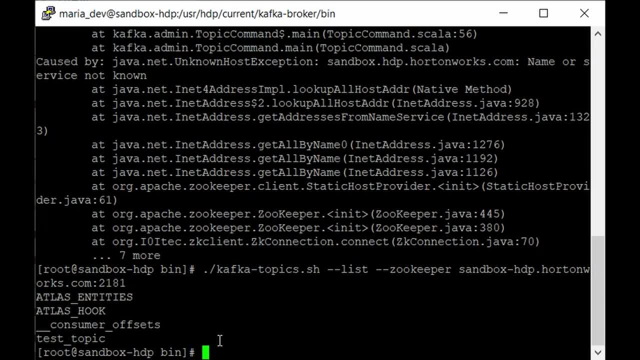 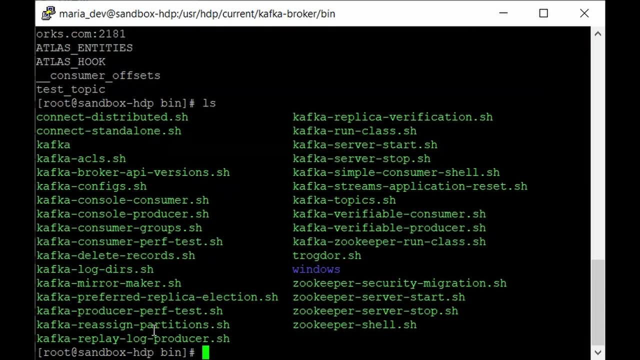 listens to our created topic, which is test topic for our incoming data. so are you ready? okay then. so producer application is also lies in the bin directory. if you give ls you will see the kafka console- producersh and kafka console- consumersh files. so first step would be to kick off the producer file to ingest some data into it. so we'll give like. 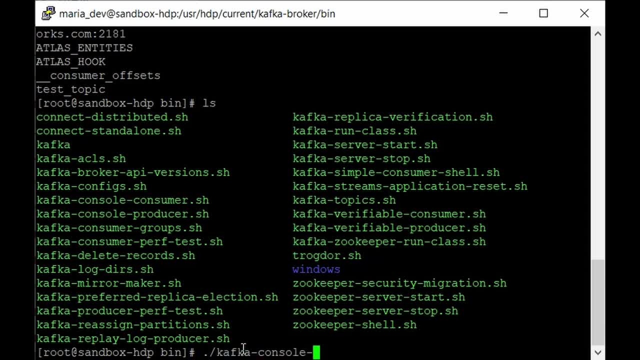 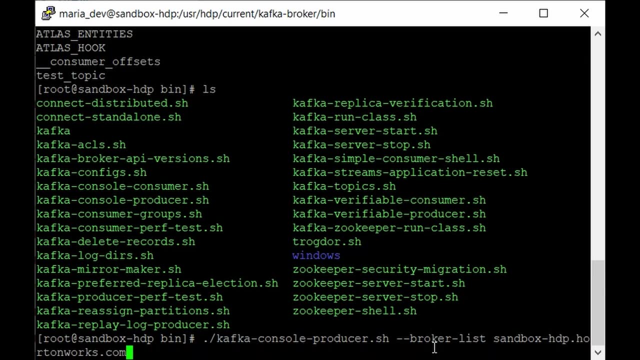 dot slash kafka dash console, dash producer dot sh. then we have to give the broker list here. so just give like broker dash list. then we have to give address for our broker which is sandbox dash, sdp dot hortonworks dot com, colon, and we need to give any port which is 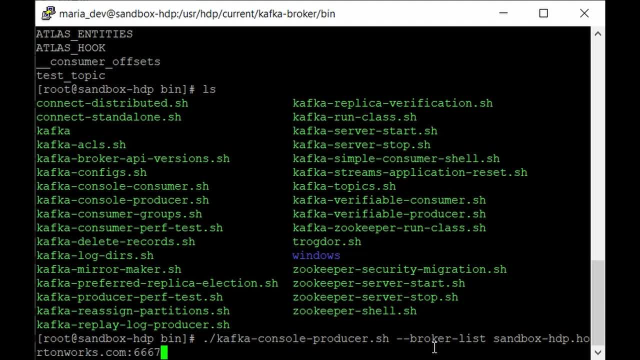 available right now. so i know that the port six, six, six seven is available right now. so we'll give the same and we have to give the topic name. so the topic name is a test topic. so if we hit enter, as you can see, we can enter any data here. so we can say like: 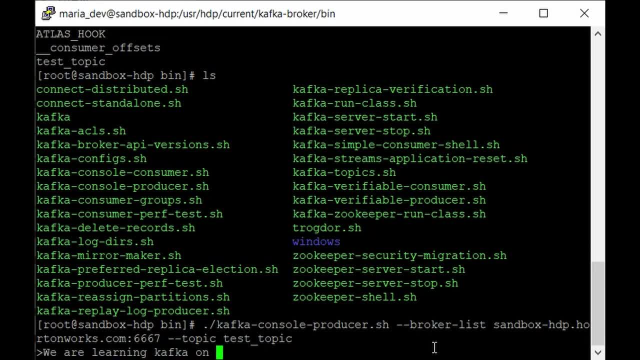 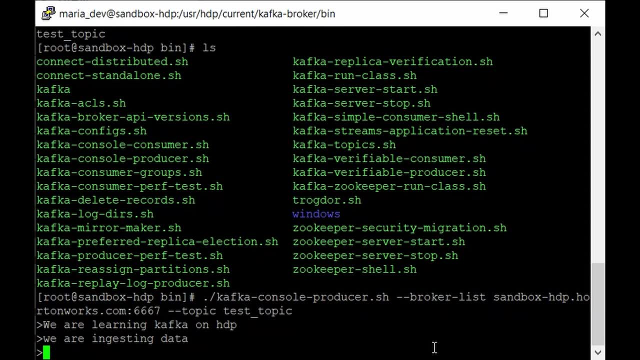 we are learning kafka on hdp. we can say we are ingesting data. so all it is doing is it is ingesting data in our test topic, but how we can validate it? i guess you guessed it correctly: we need to kick off the consumer application now. but how we can do that? so for that we'll. 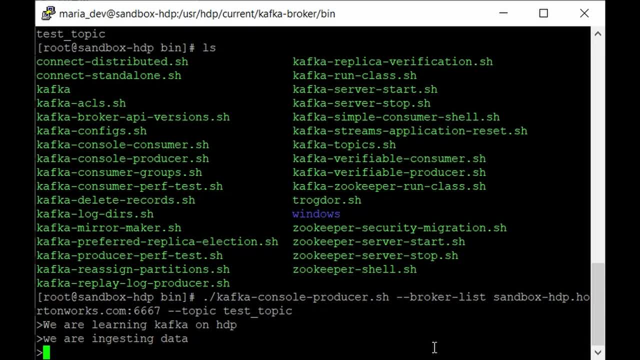 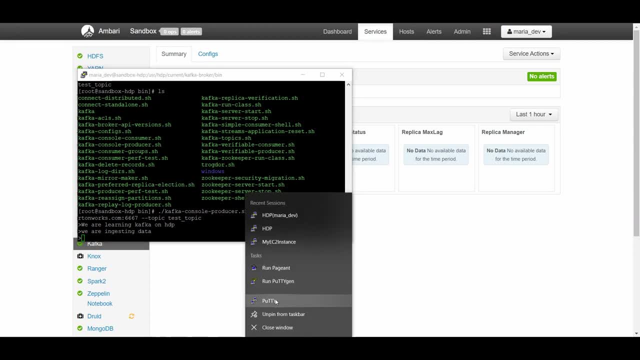 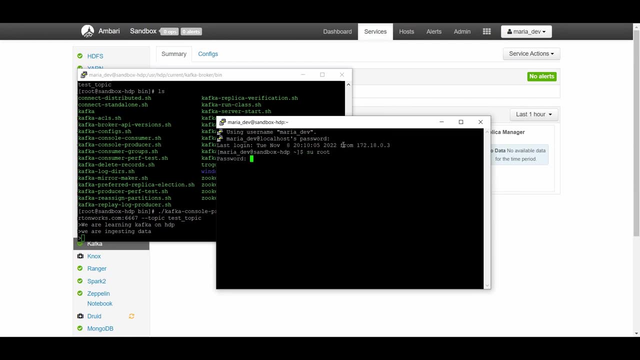 create another putty session to kick off our consumer application. okay, so we have the producer application which is running, so we'll just create new session here. so I'll just give, like mar Awards code def, login to that and again login as a root user to get you all the privileges. 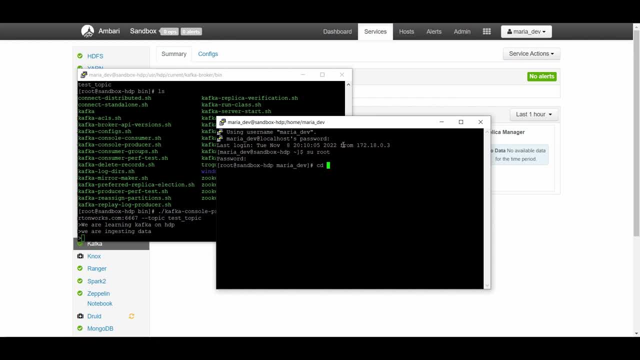 with the password and here again go to the kafka directory now. so give like user hdp, slash, current slash kafka broker and the bin directory. So now then we have to take that root user to the Kafka broker and the bin directory. give like slash bin and here, if you give ls, we have the. 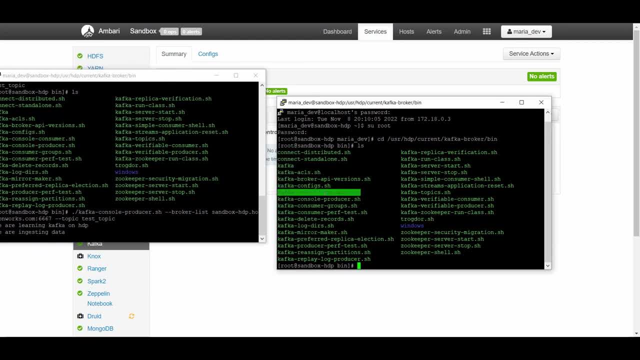 Kafka consumer application. here you can see the Kafka console consumer is here. so again, give like dot slash, Kafka console dash consumer dot sh. we need to give the zookeeper now and we don't need to pass the broker list here. but in version 2.5 we need to give the broker list and give our address. 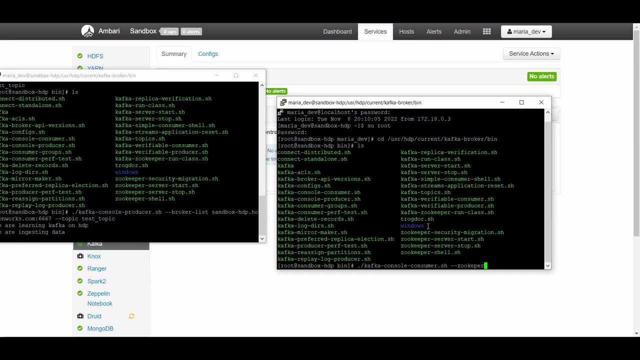 to 6667 port. but here, in version 2.6.5, we don't need to do that. we just need to give the zookeeper address, which is localhost colon 2181, as you already know, and you have to give the topic. so the topic you already know, test underscore topic and you have to pass the argument as from: 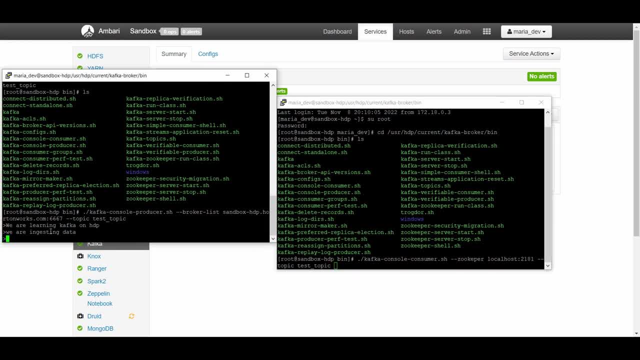 beginning, so it will also listen to the data which we have already ingested. so here we have two lines of data in our topic, and so we'll pass the argument like from dash beginning. so if you hit enter, i guess i have missed the zookeeper. e, yeah, i guess this. 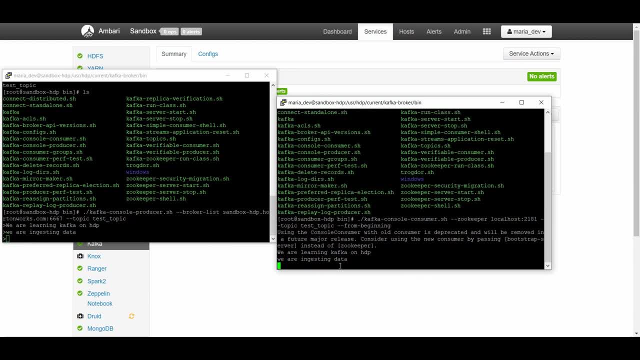 looks good. so if you kick off this, yeah, as you can see, we got the already inserted data in our topic, so let me simulate a real-time data streaming scenario. so here in one window, we have the producer script running, which is nothing but a producer application which ingests the data. 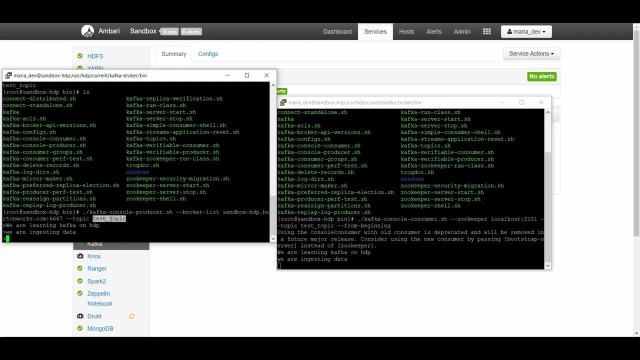 into our Kafka topic. so here our Kafka topic is the Kafka topic, and we have the Kafka topic is test underscore topic, and here we have the consumer application which consumes the data. so this is not a very high level thing. this is just to let you know how it works under the hood. 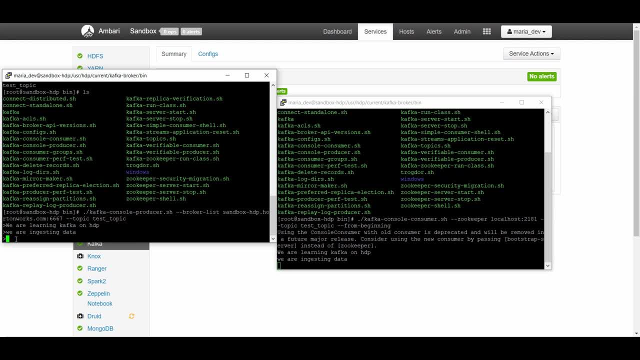 and we are just ingesting some text data, but in real world scenario, you'll be getting millions of rows every hour in real time, which are, which could be coming from iot devices or any sensors, or coming from any social media websites, and you have to process it in real time. 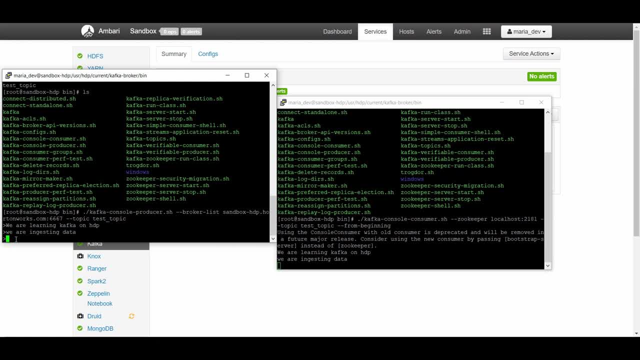 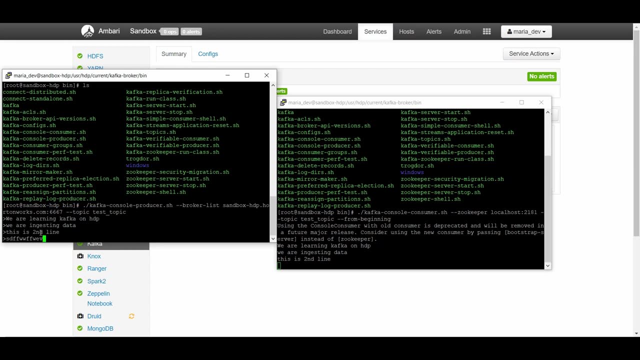 so that's where kafka is so powerful and backbone of big companies like linkedin and netflix. so, if you just give like, this is second line and, as you can see, we got the message in just a second. also, if you can give like any raw data, as you can see, so we are getting all this data in real time. 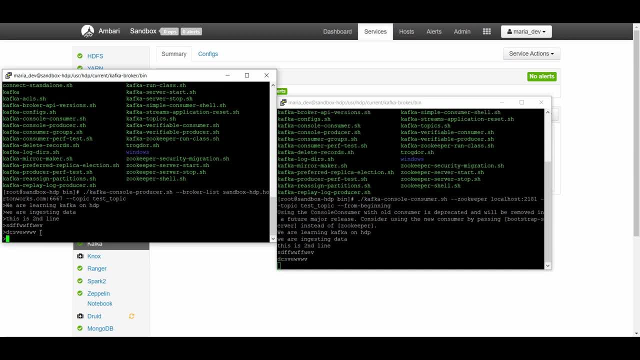 so this is just to let you know the power of kafka. so we are ingesting the data from one end and consuming it from the other end. so this is how kafka works under the hood and how we can simulate a real-time data streaming platform by using this service. so this was just a basic demo from the command line, but in the